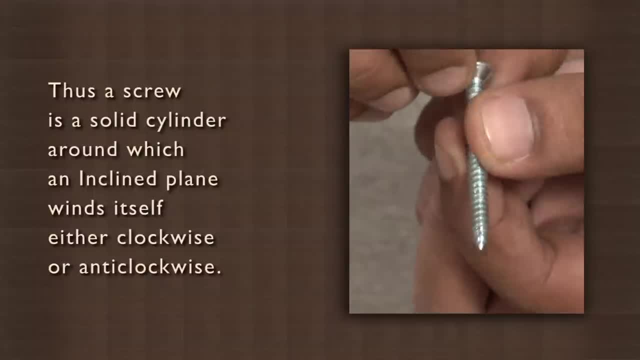 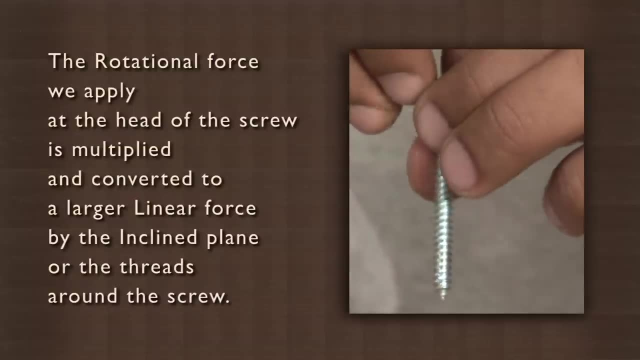 Thus, a screw is a solid cylinder around which an inclined plane winds itself, either clockwise or anticlockwise. The rotational force we apply at the head of the screw is multiplied and converted to a larger linear force by the inclined plane or the threads around the screw. 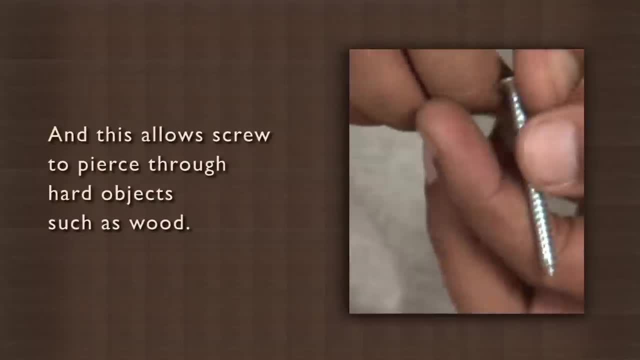 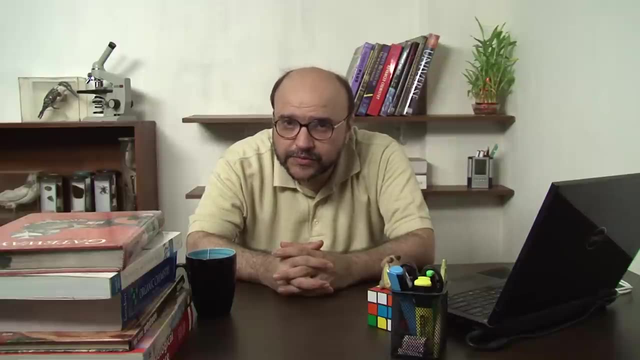 And this allows screw to pierce through hard objects such as wood. Majority of bottles, you will see, will have a screw cap lid, which is also an example of a screw. 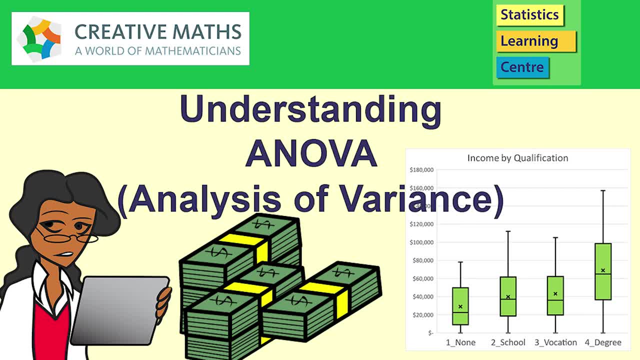 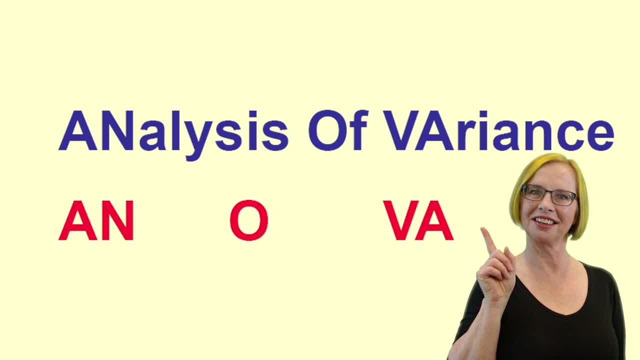 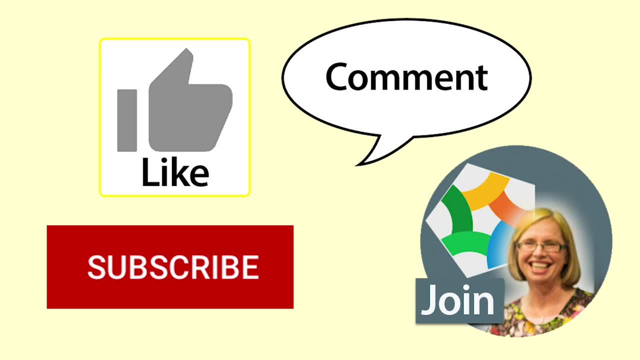 Understanding ANOVA, or Analysis of Variance. Hi, I'm Dr Nic and in this video I'm going to tell you about Analysis of Variance, or ANOVA. Before we start, please like this video, comment below, subscribe, but, most of all, join the channel, Help it grow and help me help more and more people like 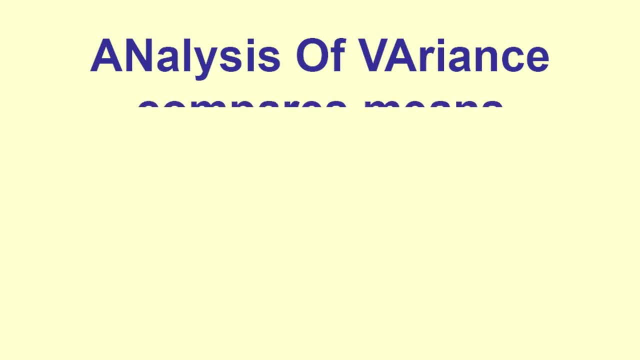 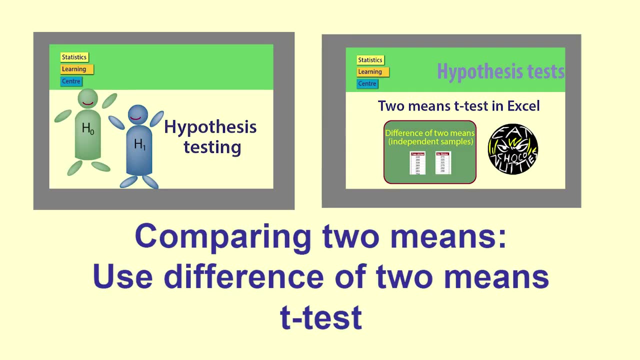 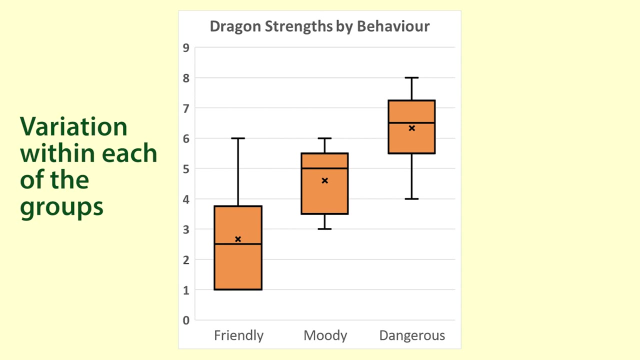 you, Analysis of Variance is used to compare means. When we compare two means, we generally use a t-test for the difference of two means, But when we have more than two groups that we are comparing, we need to use ANOVA. We calculate the variation within each of the groups and 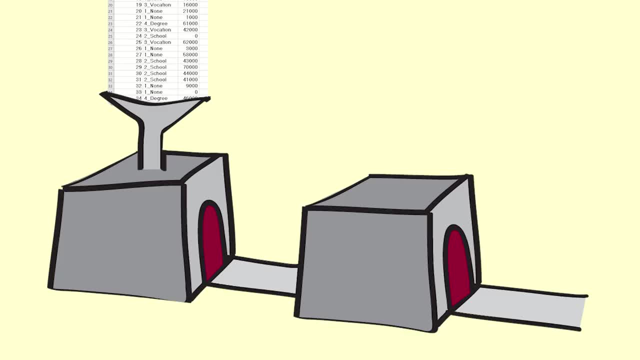 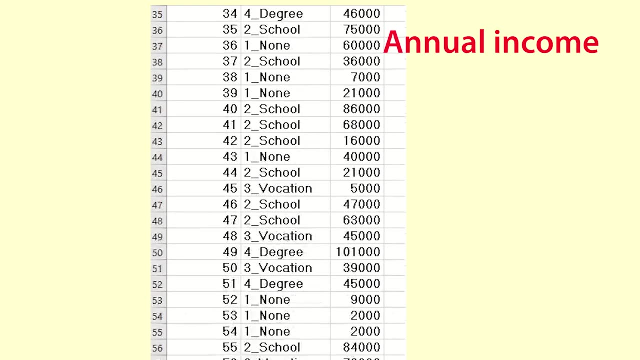 compare it with the variation between the groups. This is usually done using a computer program. The f-statistic is calculated, which is compared with the f-distribution, and from that the computer provides a p-value. Here is an example based on real data about people's annual incomes. 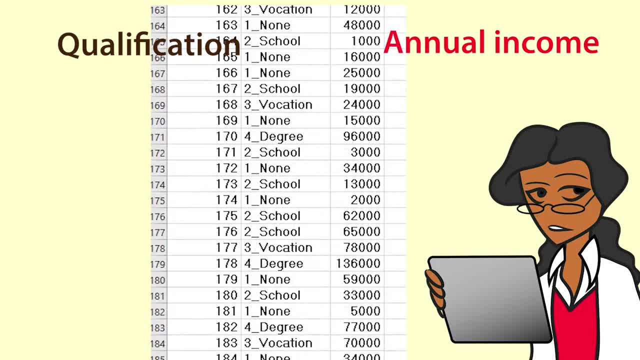 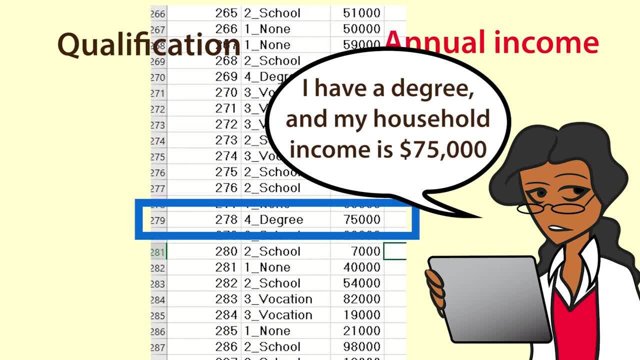 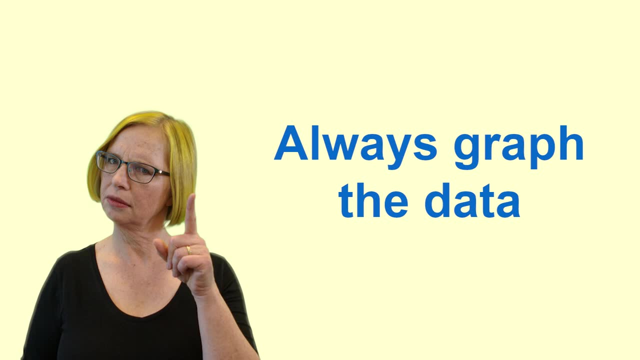 and income. Here is an example based on real data about people's annual incomes and income. For each person, we have data about their level of qualification and their annual household income. We would expect there to be a difference in income depending on level of qualification. Remember always graph the data. I have used Excel to create. 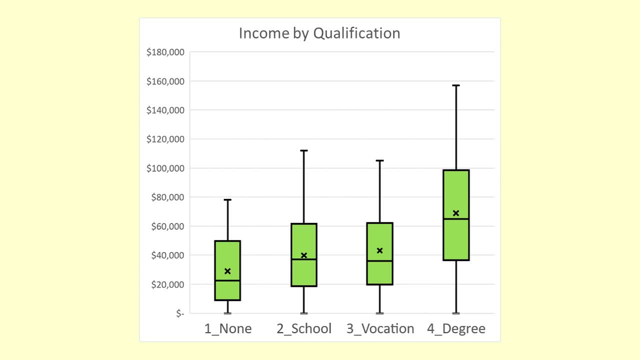 comparative box and whisker plots for the different qualification groups. This helps us to see what is happening in this sample. You can see that in the sample, people with degrees tended to earn more than those without degrees. The other means look similar to each other.